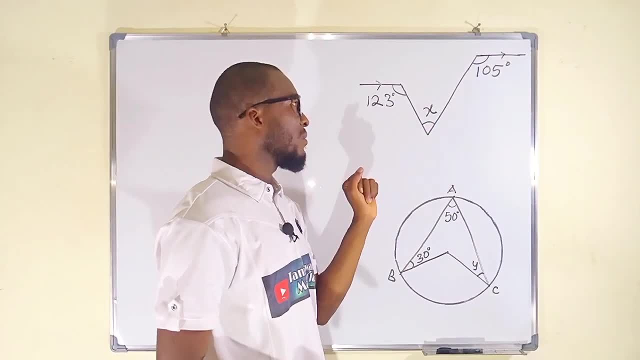 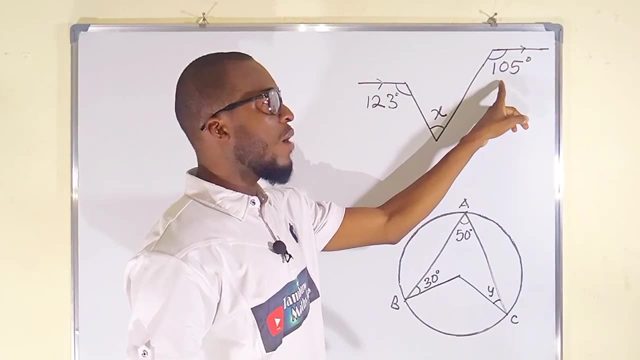 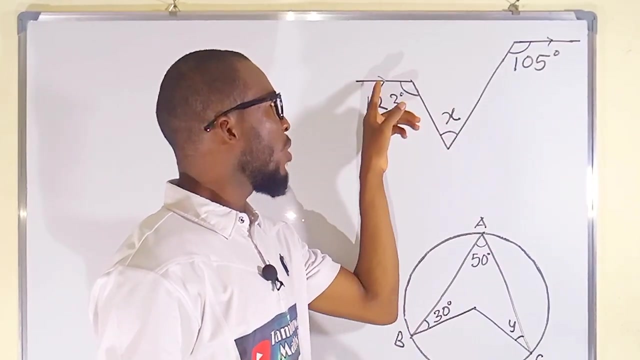 We want to find this angle, which is represented by x. But let us observe the diagram carefully. We have 123 degrees here and we have 105 degrees here. But of that, these two lines, they are parallel to each other. This is why we have these two marks indicating that no matter. 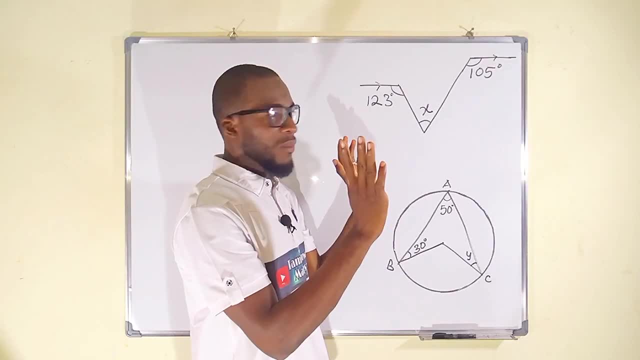 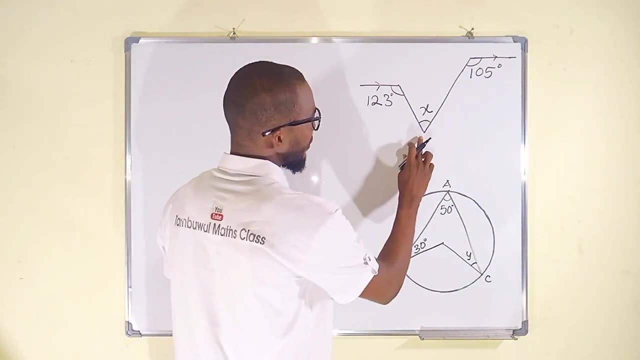 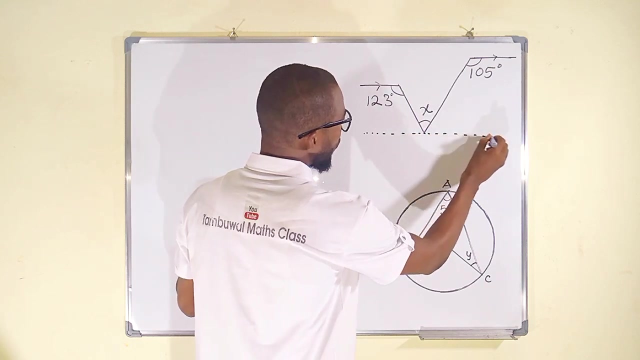 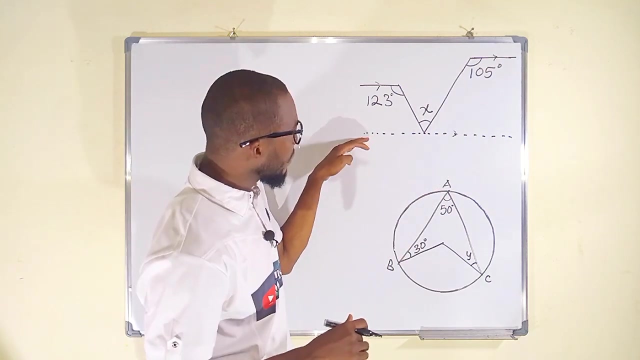 where they get to. they will never meet. So therefore they are parallel. So now we can construct an imaginary parallel line just beneath this angle, So such that it will be parallel to the two lines this and this. So this should also have a mark here. What does this mean? It means that 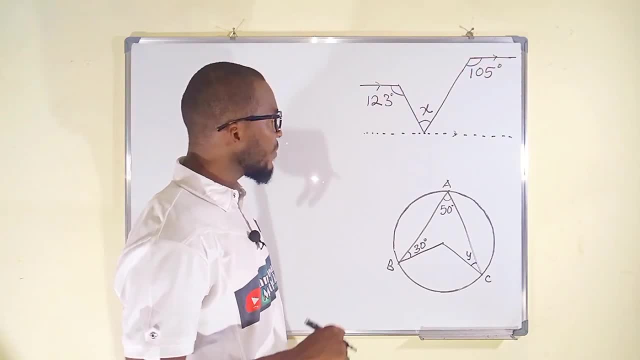 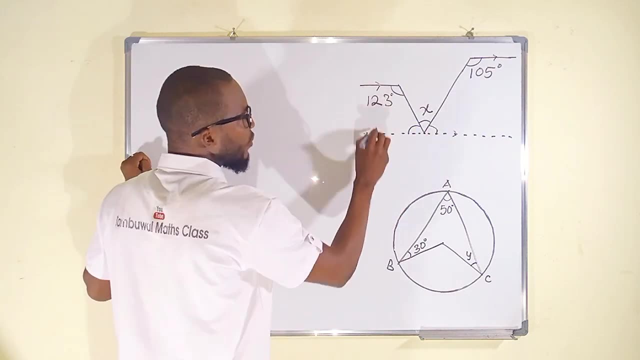 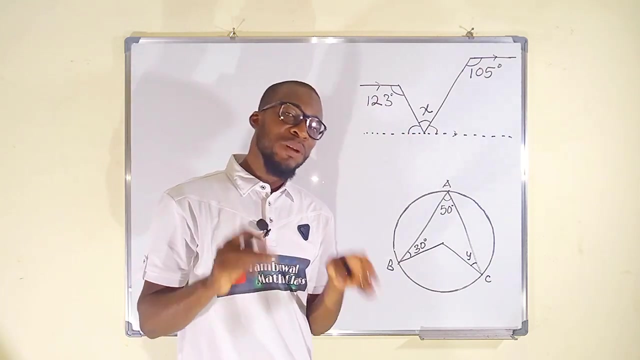 this line is also parallel to these two lines. All right, let us observe this: This angle here and this other one. Remember, if these two lines are parallel to each other, this angle and this angle are said to be supplementary. If they are supplementary, 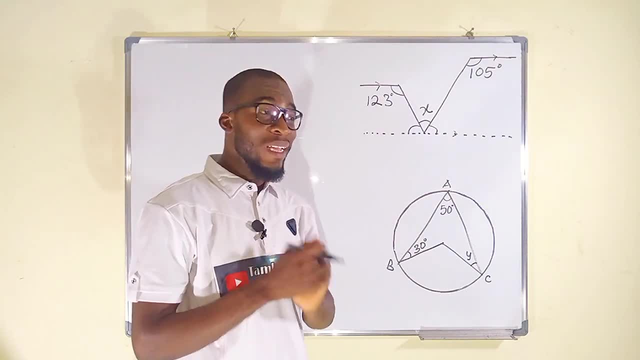 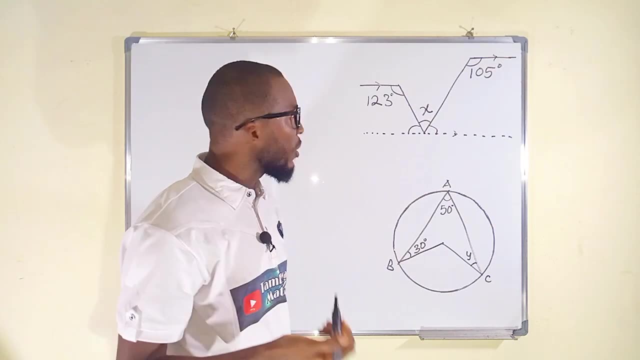 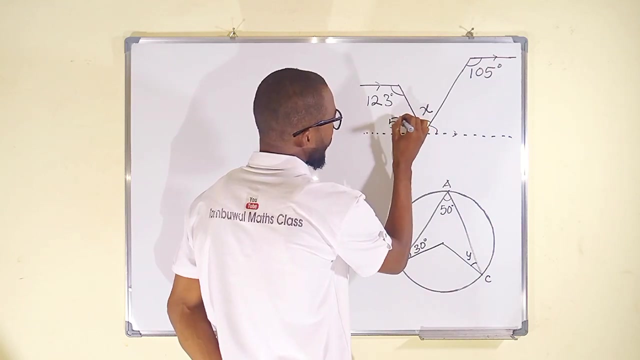 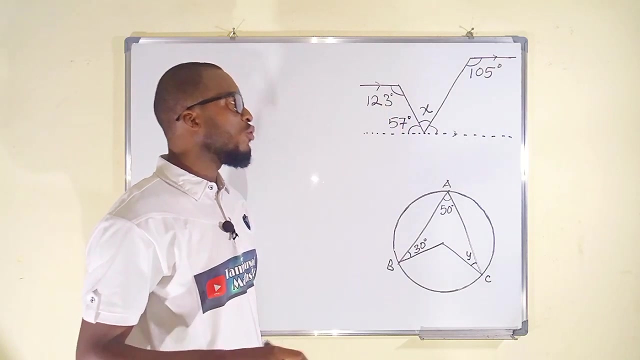 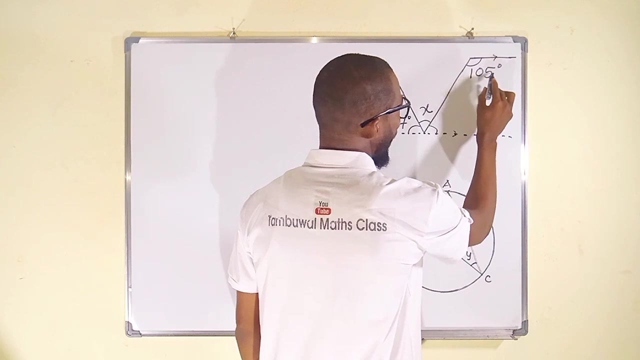 this plus this will be equal to 180.. So to find this angle, we can just subtract 123 from 180, which is going to make it 57. Because 123 plus 57 is equal to 180.. Likewise, here, 105 plus 75 will be equal to 180, because 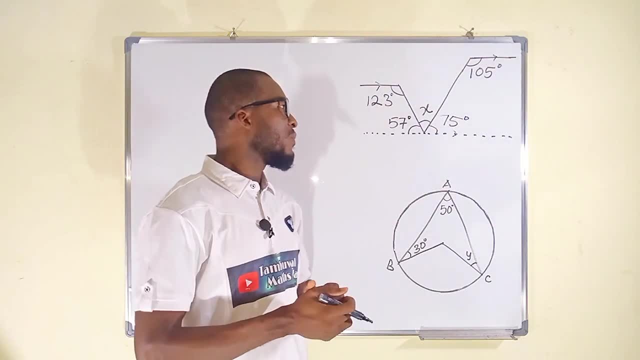 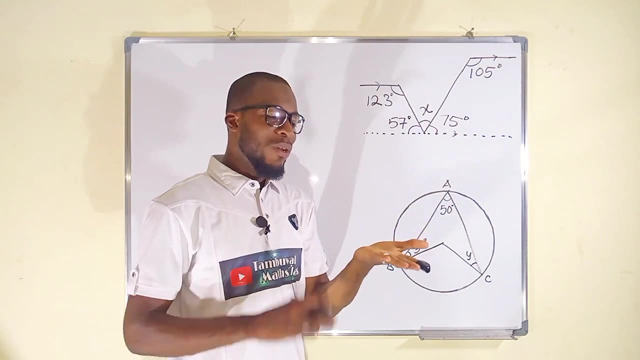 these two angles are also supplementary. Now we are good to go to find the value of x. Remember, this is a straight line. An angle on a straight line is equal to 180.. This means that if we add these three angles together, 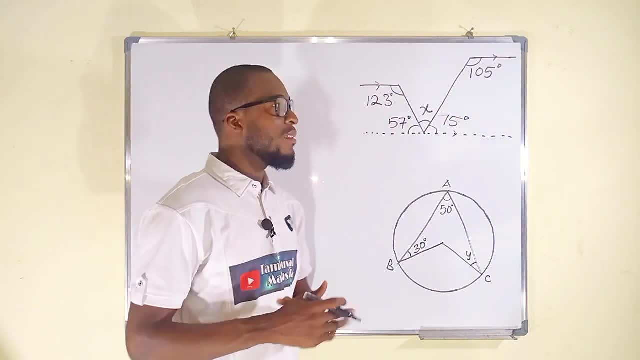 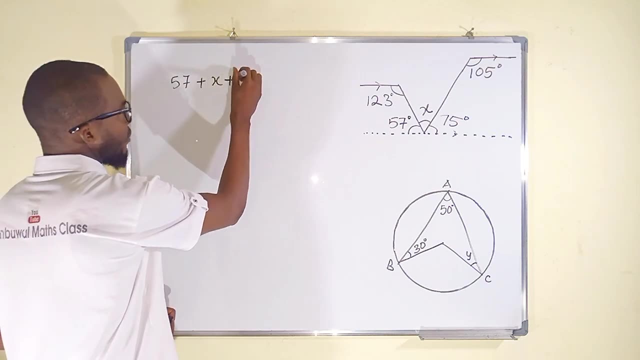 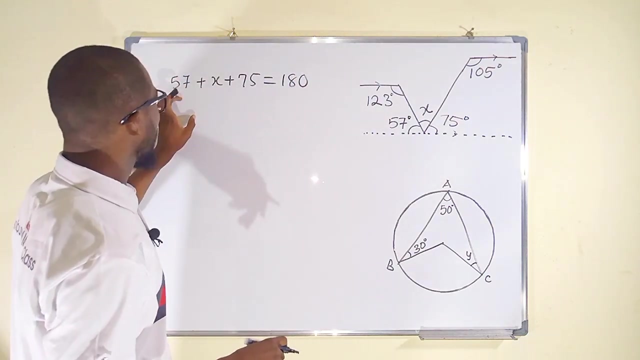 one, two, three, we are going to obtain 180 degrees. So we can do it here: 57 plus x plus 75 is equal to 180.. What we are going to do next is to take all these numbers to the right. 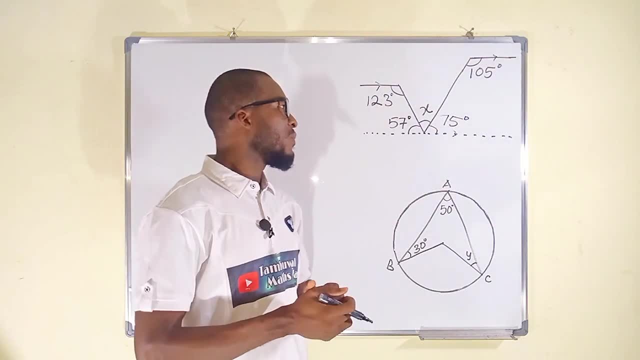 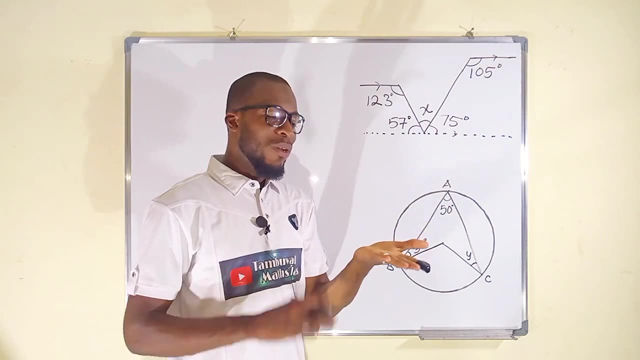 these two angles are also supplementary. Now we are good to go to find the value of x. Remember, this is a straight line. An angle on a straight line is equal to 180.. This means that if we add these three angles together, 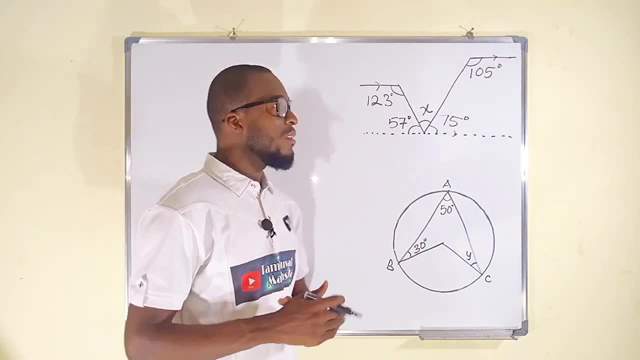 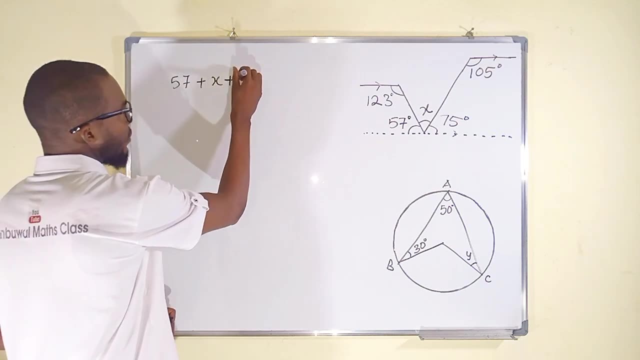 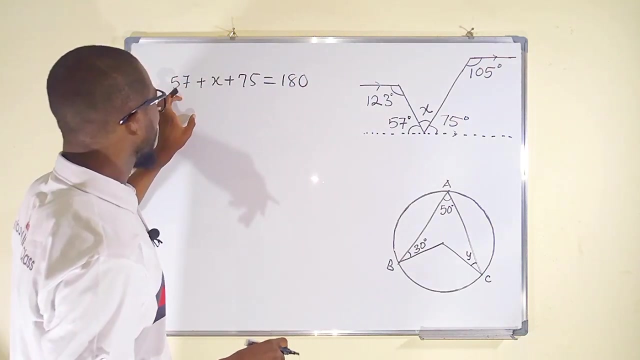 1,, 2, 3, we are going to obtain 180 degrees. So we can do it here. 57 plus x plus 75 is equal to 180.. What we are going to do next is to take all these numbers to the right. They are positive here. 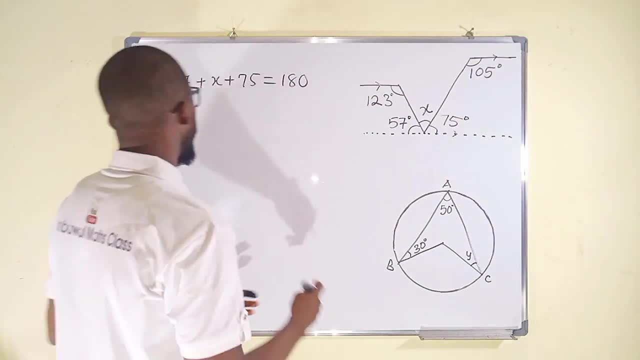 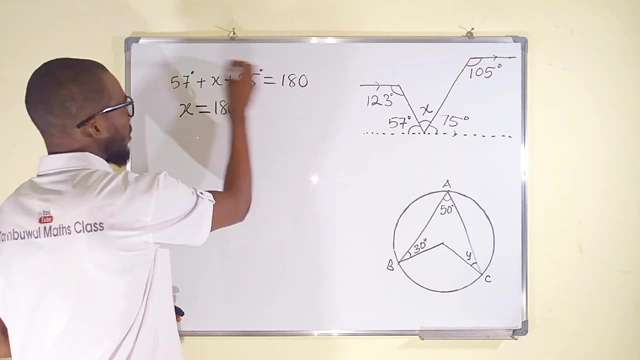 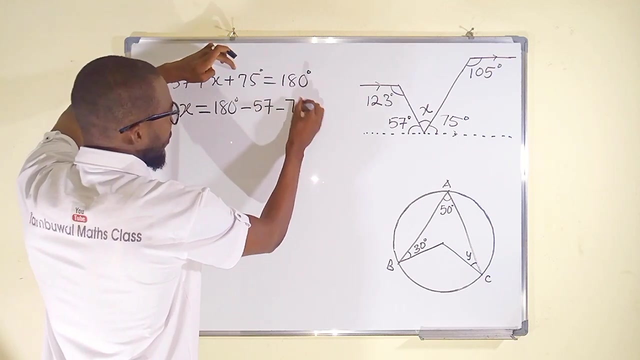 Once they cross over the equality sign, they turn to negative, leaving only x to the left. x now equal to 180. remember: all these values are in degrees minus. we have 57 here minus 75. they're all in degrees and finally, we can now obtain the. 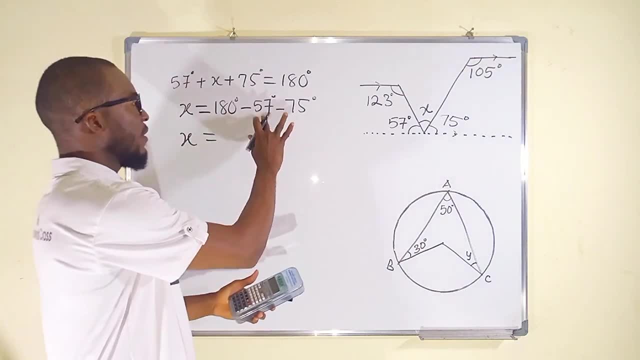 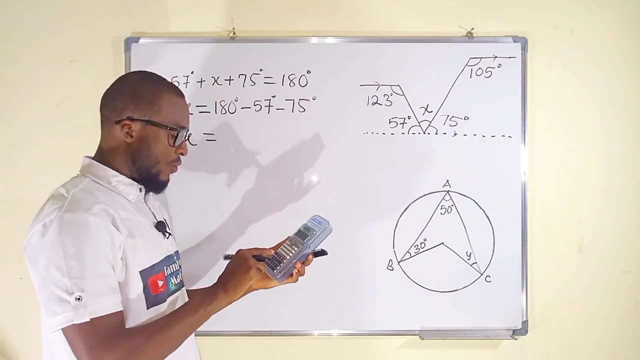 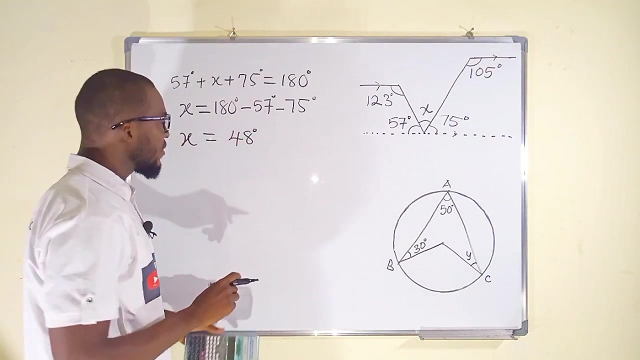 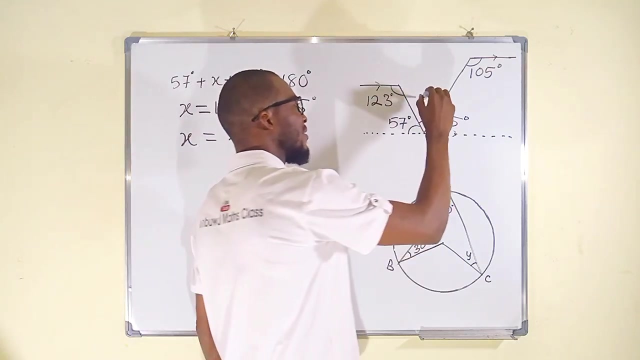 value of x. by subtracting these two from 180, we have 180 minus 57, minus also 75, and what we have is 48, 48 degrees. what does this mean? it means that this angle here which is missing, is equal to 48 degrees, and hence we say: this is equal to 48 degrees, this angle right here. 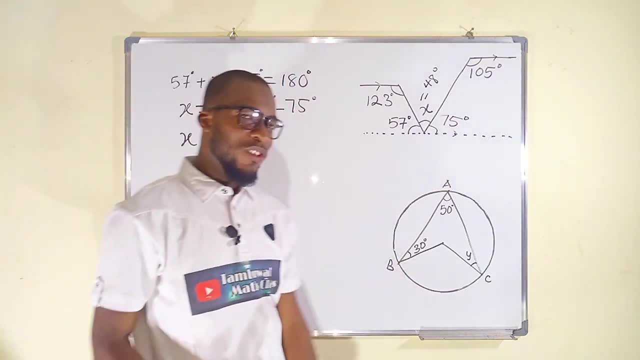 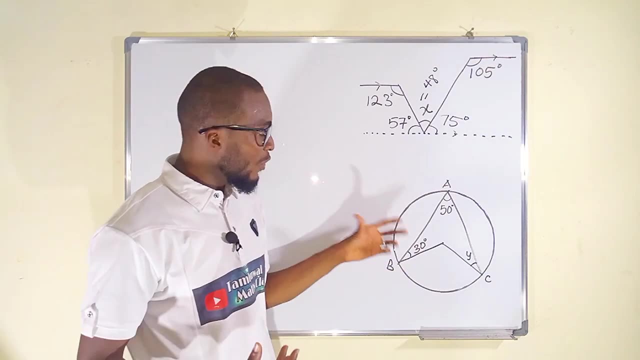 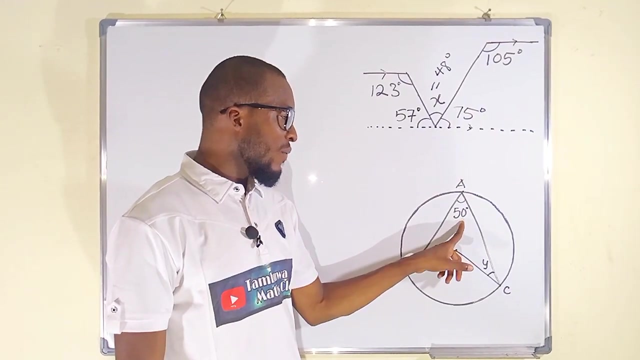 so we have answered this first question. let us move on to the second one, which is under cycle theorem. okay, the second problem is under cycle theorem, we want to find this angle here, which is represented by y. this angle, a is given as 50 and will be is given as 30. but we are looking. 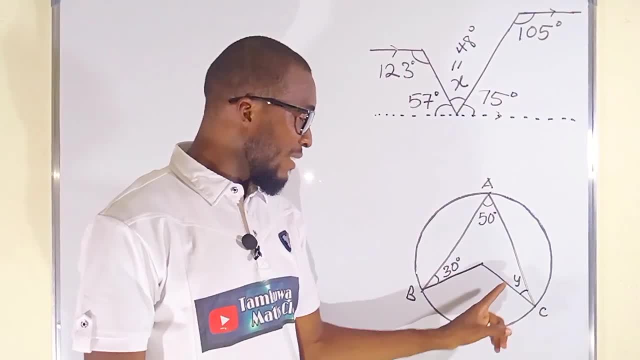 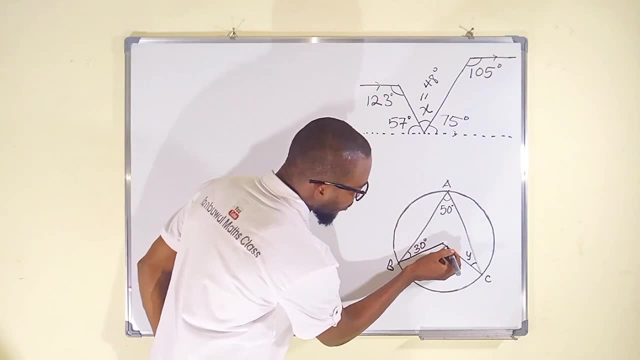 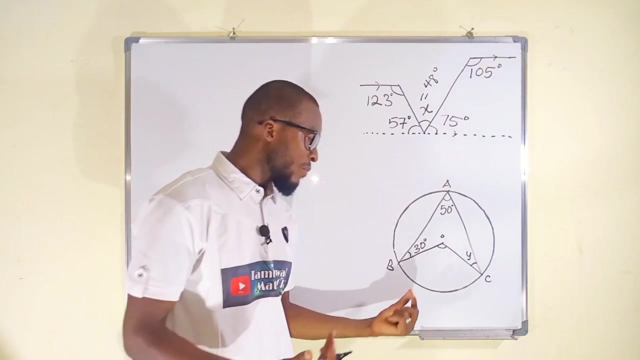 for the angle c. do not think that it is also 30 degrees. we don't know. we have to find out. you, the very first thing we need to find is this angle here. remember, this is the center. we need to find this angle here. and how can we find it? for cycle theorem, angle formed at the center is twice angle. 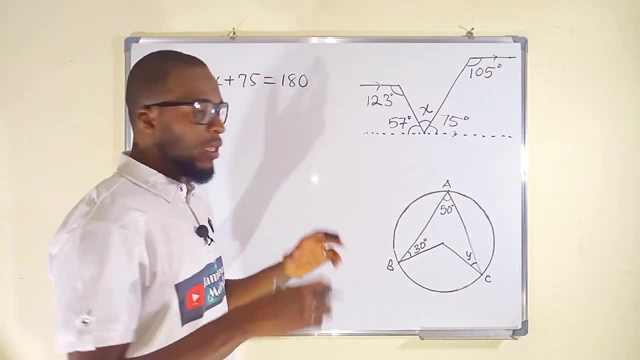 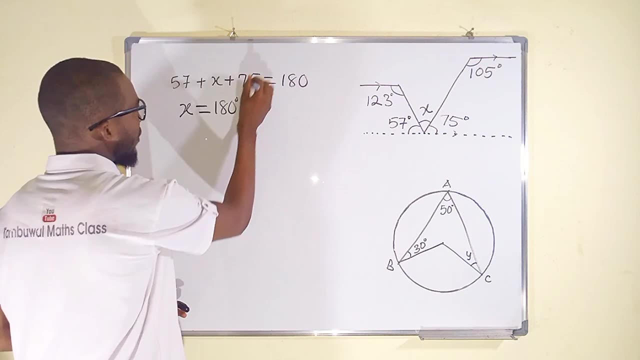 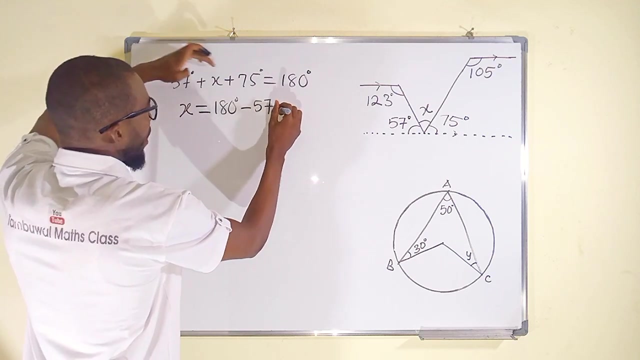 They are positive here. Once they cross over the equality sign, they turn to negative, leaving only x to the left. x now equal to 180.. Remember: all these values are in degrees Minus. we have 57 here Minus 75.. They are all in degrees. 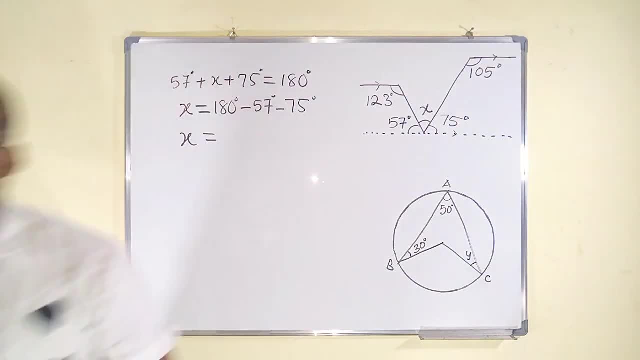 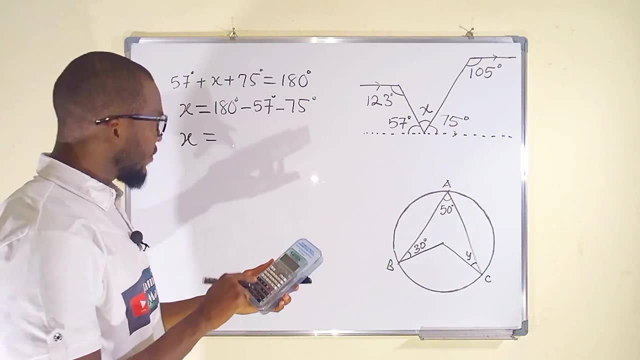 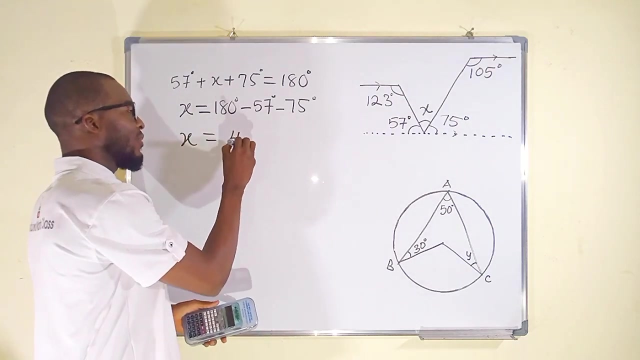 And finally, we can now obtain the value of x by subtracting these two from 180.. We have 180 minus 57.. Minus also 75. And what we have is 48.. 48 degrees. What does this mean? It means that this angle here. 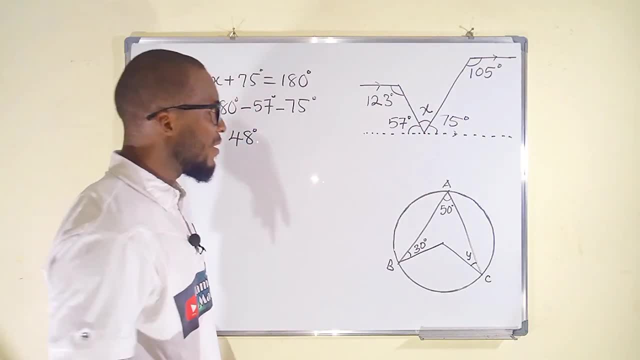 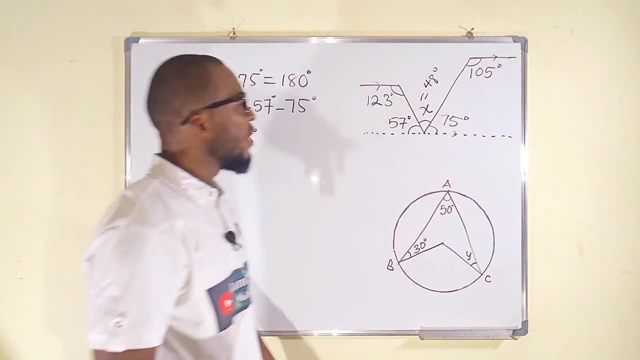 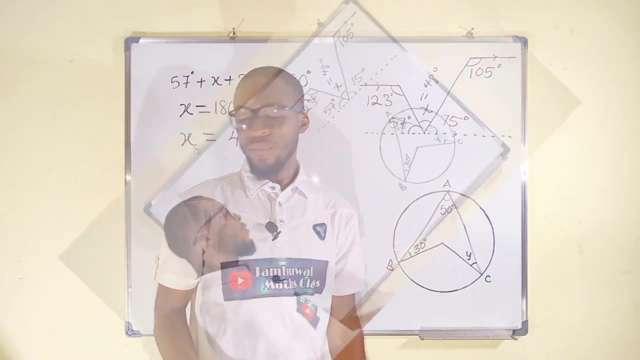 which is missing is equal to 48 degrees, And hence we say: this is equal to 48 degrees, this angle right here. So we have answered this first question. Let us move on to the second one, which is on the cycle theorem. 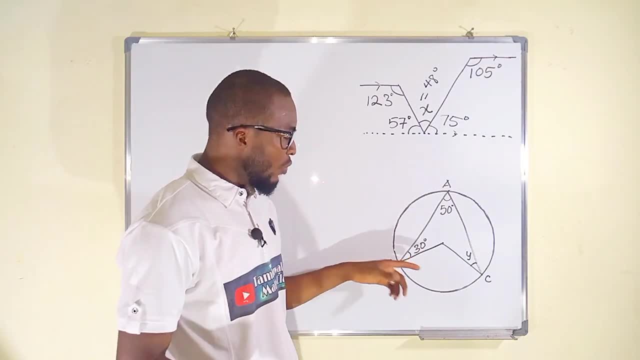 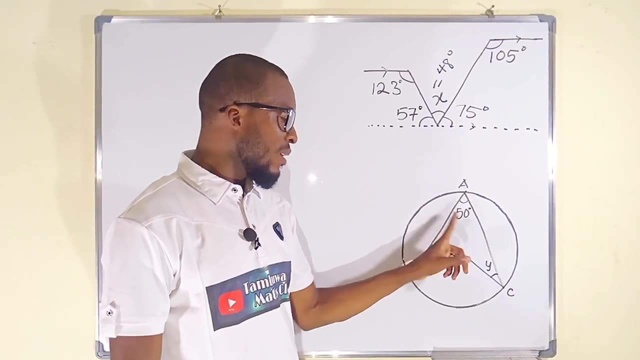 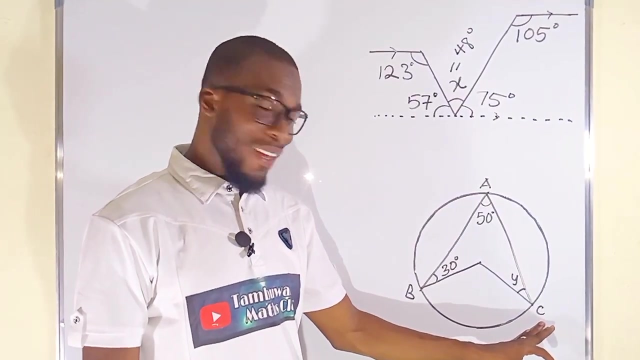 Okay, The second problem is on the cycle theorem. We want to find this angle here which is represented by y. This angle a is given as 50. Angle b is given as 30. But we are looking for the angle c. Do not think that it is also 30 degrees. We don't know. We have to find out. 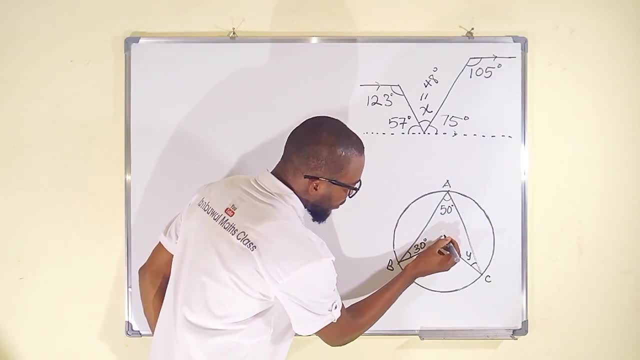 The very first thing we need to find is this angle here. Remember, this is the center. We need to find this angle here. And how can we find it? For the cycle theorem, angle formed at the center is twice angle formed at the circumference. 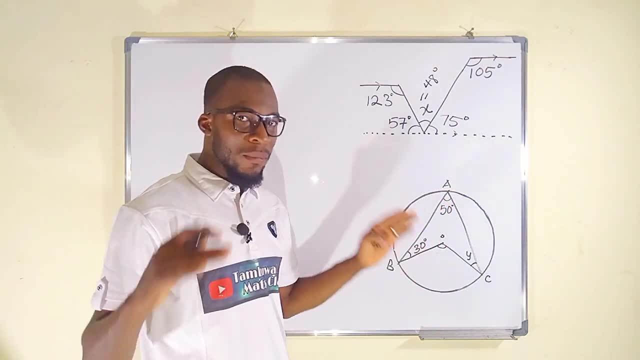 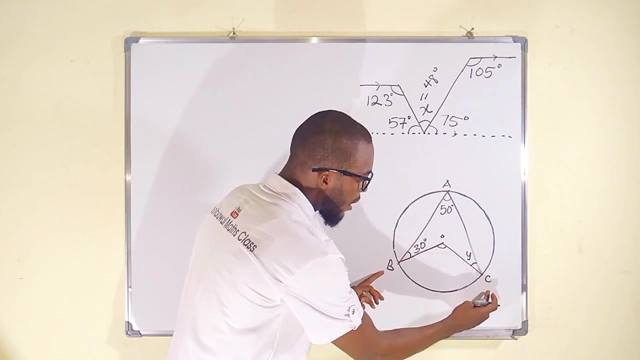 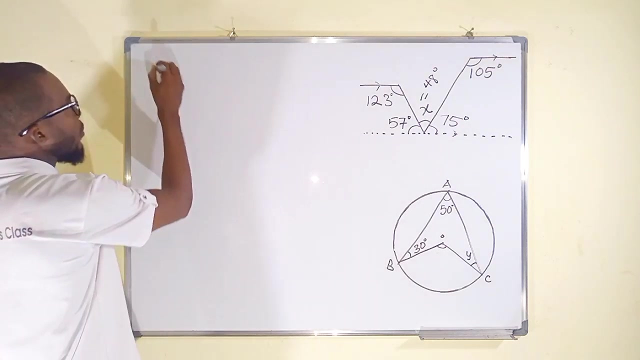 if, and only if, the two angles are formed from the same arc. You can see we have an arc bc here. This arc forms this angle to the center. likewise forms another one to the circumference. So to find this angle, we can say that, okay, angle b o c. 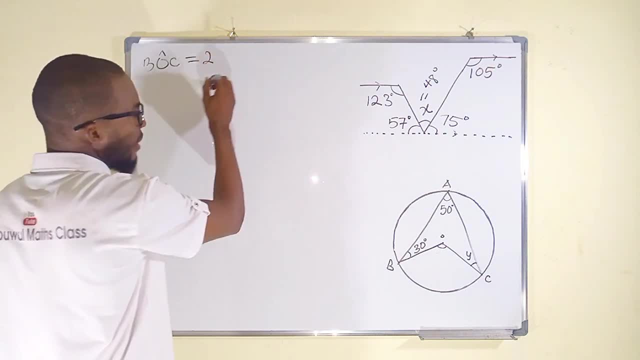 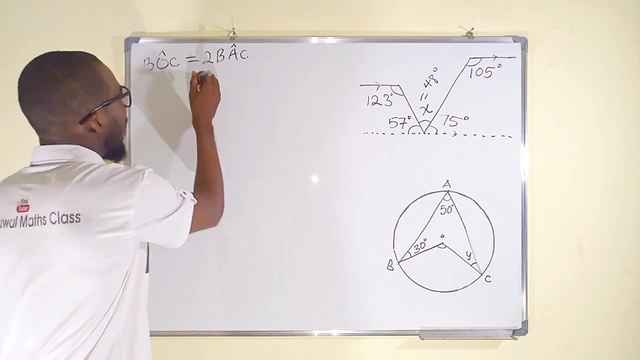 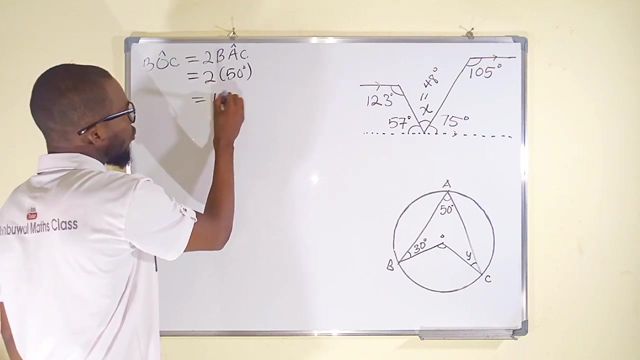 that is the name- is twice, two times the angle formed to the circumference, which is b, a, c, And this is equal to 2 multiplied by 50, because that angle is 50 degrees And this is equal to 100 degrees. 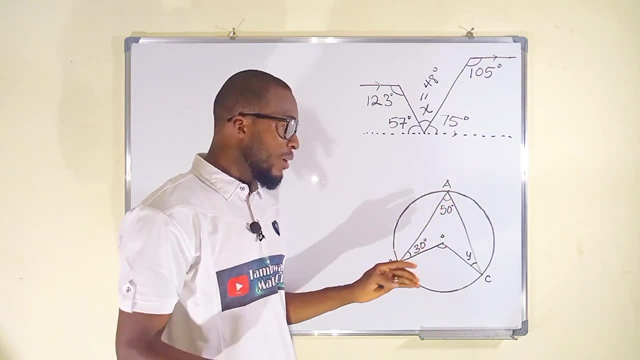 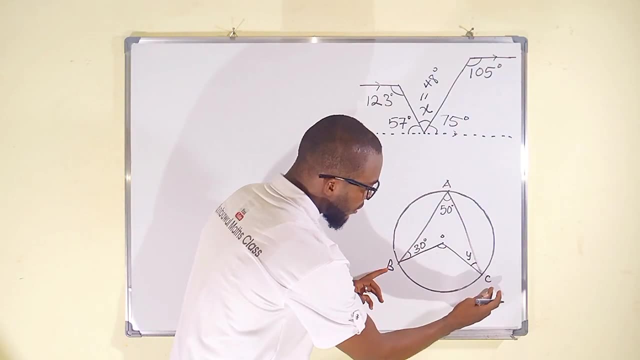 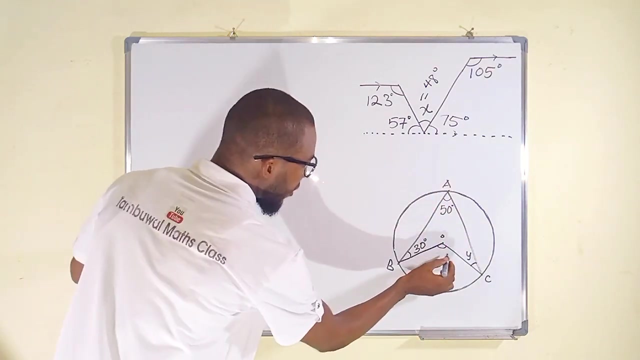 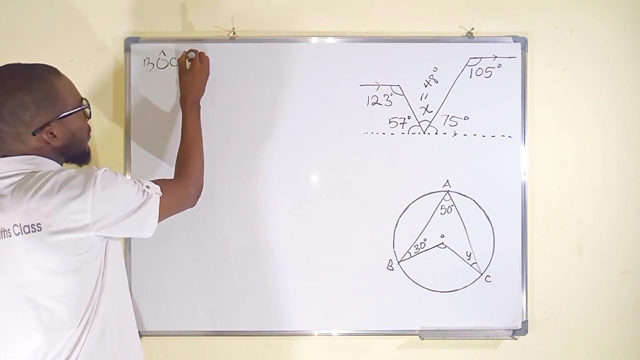 formed at the circumference, if, and only if, the two angles are formed from the same arc. you can see, we have an arc bc here, this arc from this angle to the center, likewise from an hour to the circumference. so to find this angle, we can say that, okay, angle b o c, that is the name. 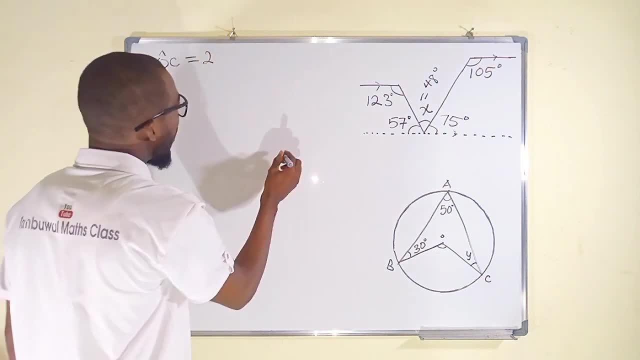 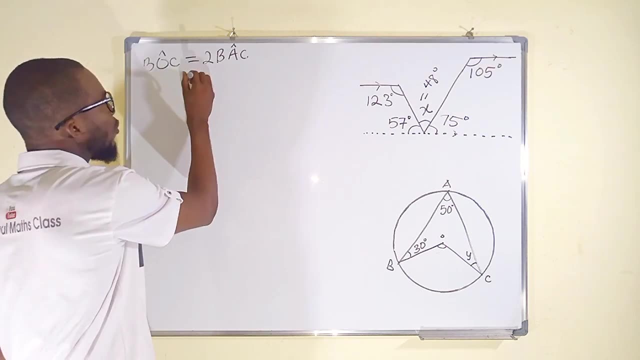 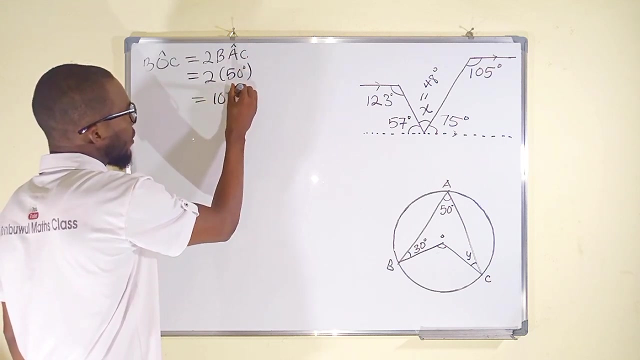 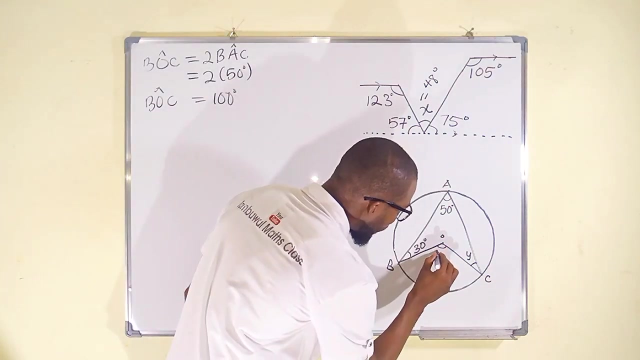 is twice, two times the angle formed to the circumference, which is b a a c, and this is equal to 2 multiplied by 50, because that angle is 50 degrees and this is equal to 100 degrees. so b o c is equal to 100 degrees. this angle right here is 100 degrees. what do we do next? we can construct an. 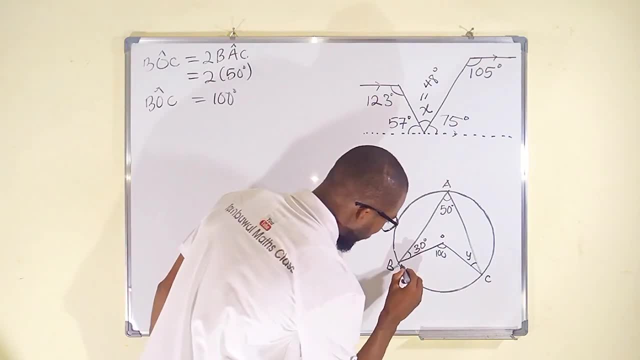 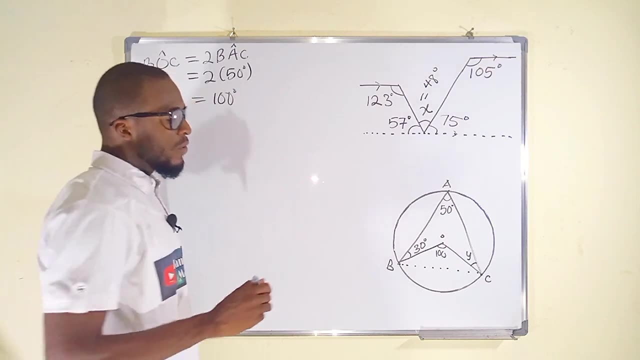 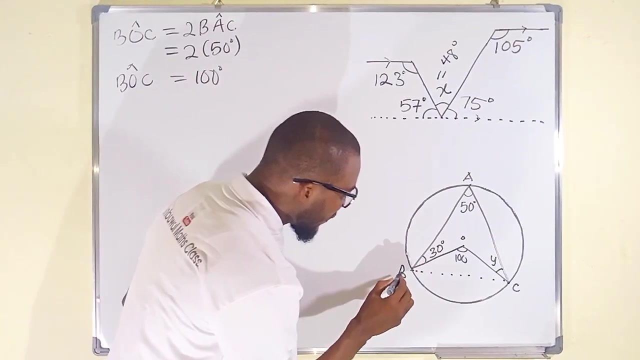 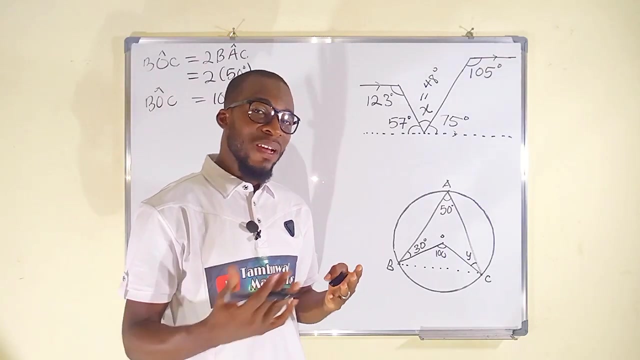 imaginary straight line connecting b and c. remember i told you the way i will solve it might be entirely different from the way you will solve it. so this imaginary line connecting b and c form an isosceles triangle. so this triangle b o c is an isosceles triangle. remember, an isosceles triangle is that type of triangle in which 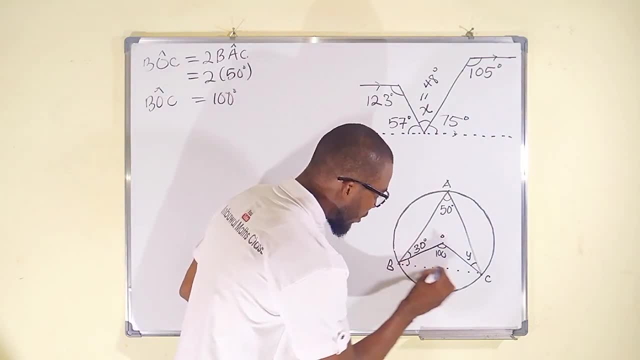 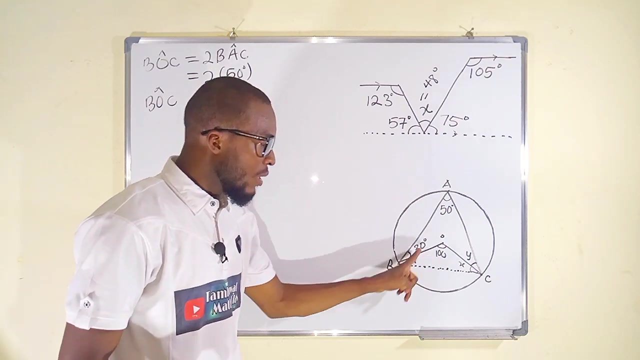 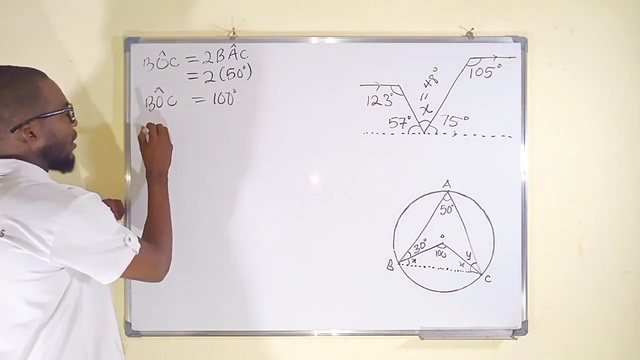 the base angles are exactly the same, so this angle here and this angle here are the same. so if this is x, this must be x, because they are the same. but we know that the total angle in a triangle is 180 degrees. so now we can find this value of x. x plus x plus 100 is equal to 180.. x and x is 2x and you have to take. 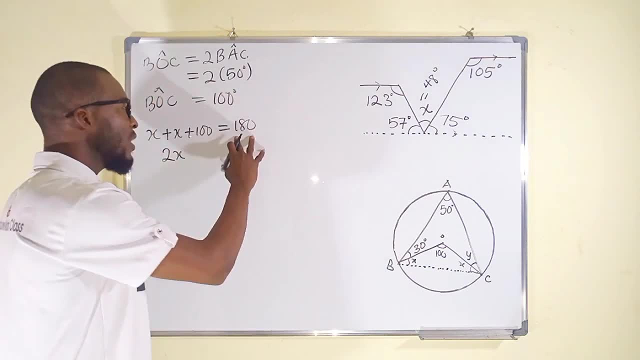 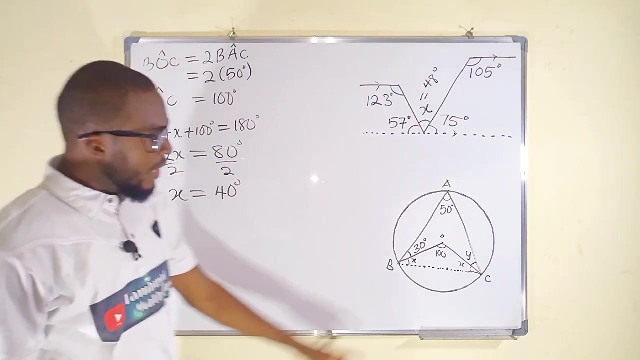 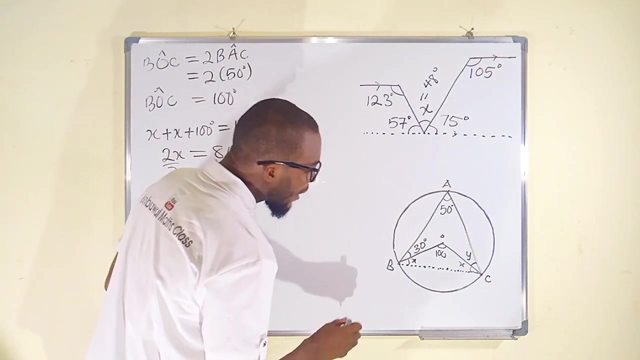 100 to the right and it becomes negative. we have 180 minus 100, which is equal to 80.. divide both sides by 2 to obtain the value of x, and x finally is equal to 40 degrees. it means that each of these angles equals 40 degrees. all right, look at, we have another triangle. 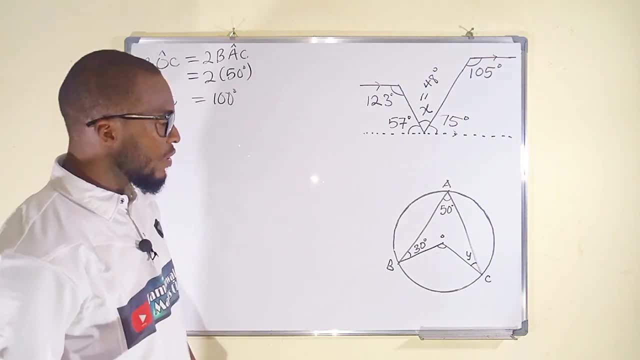 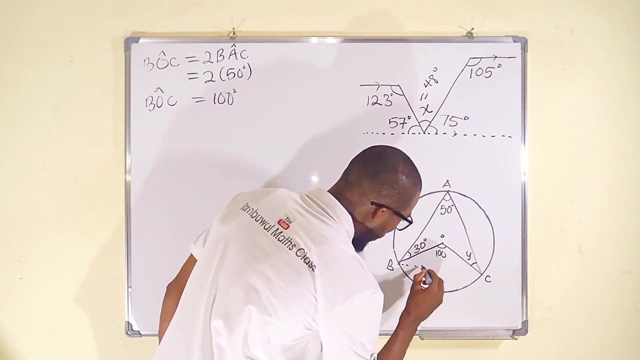 So b o c is equal to 100 degrees. This angle right here is 100 degrees. What do we do next? We can construct an imaginary straight line connecting b and c. Remember I told you the way I will solve it might be entirely different from the way you will solve it. 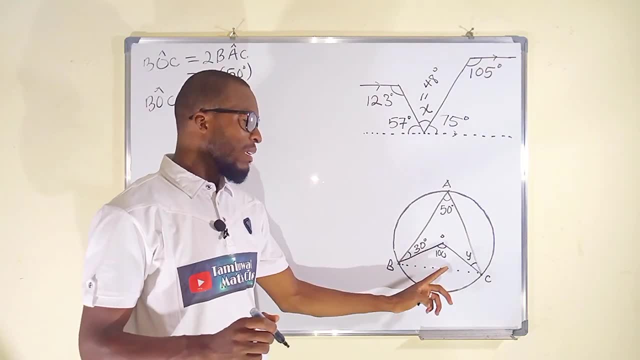 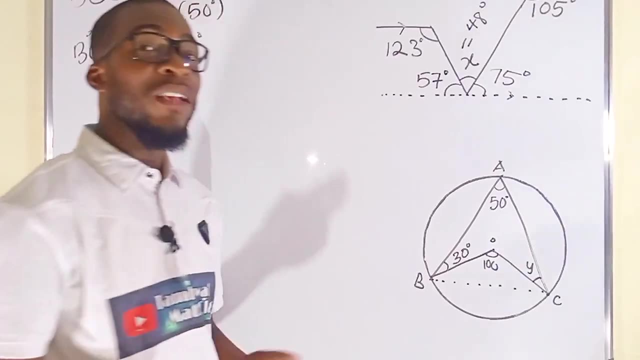 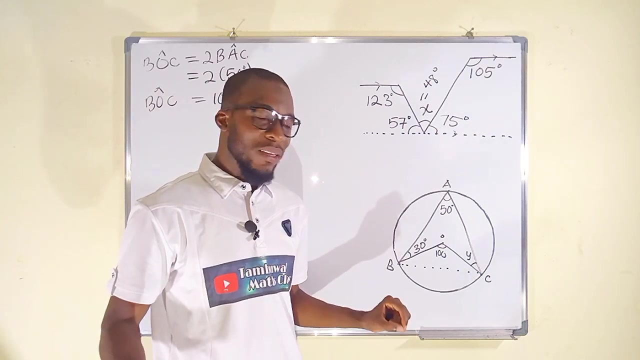 So this imaginary line connecting b and c form an isosceles triangle. So this triangle b o c is an isosceles triangle. Remember, an isosceles triangle is that type of triangle in which the base angles are exactly the same. so this angle here and this angle here are 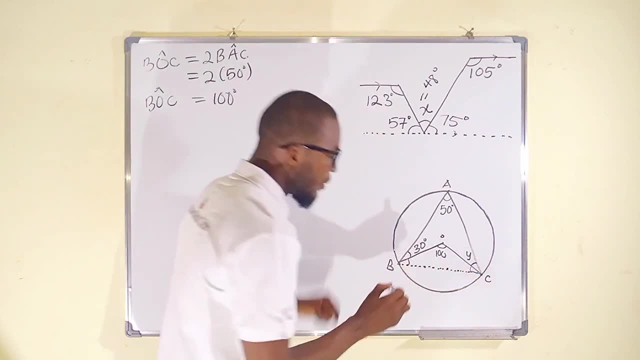 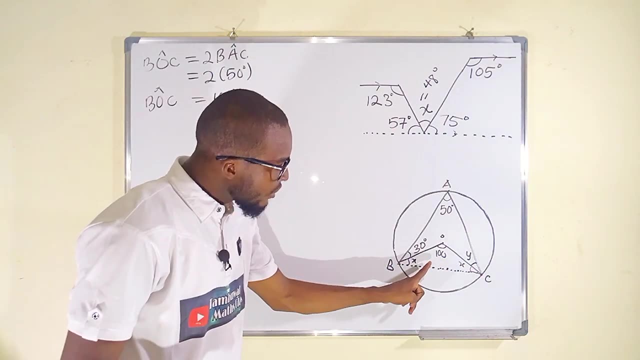 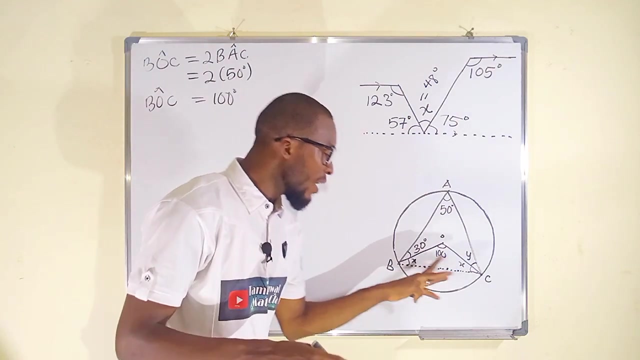 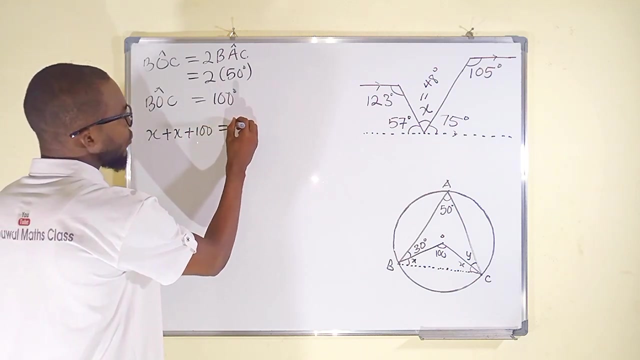 the same. so if this is X, this must be X, because they are the same. but we know that the total angle in a triangle is 180 degrees. so now we can find this value of X. X plus X plus 100 is equal to 180 X and X is 2 X and you have to take 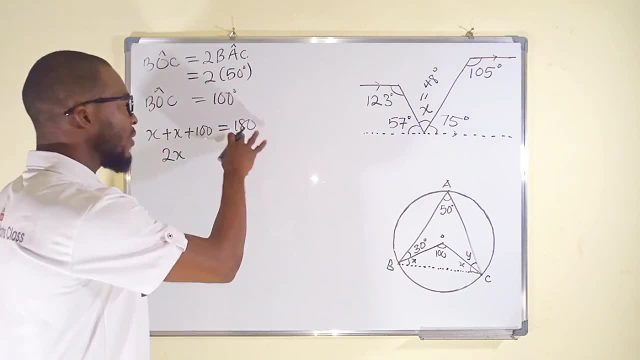 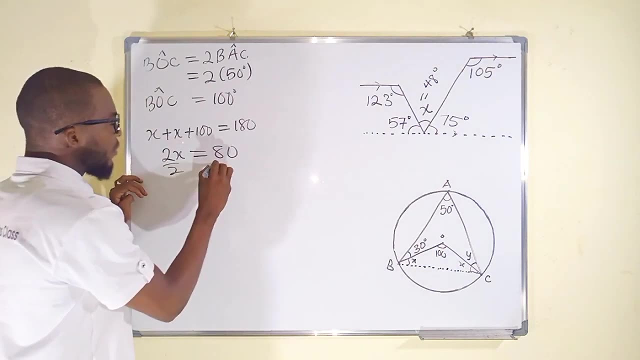 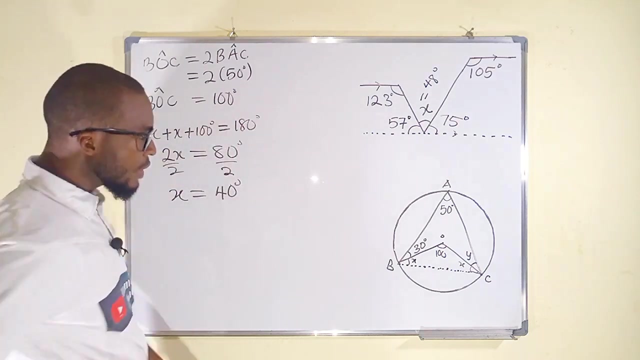 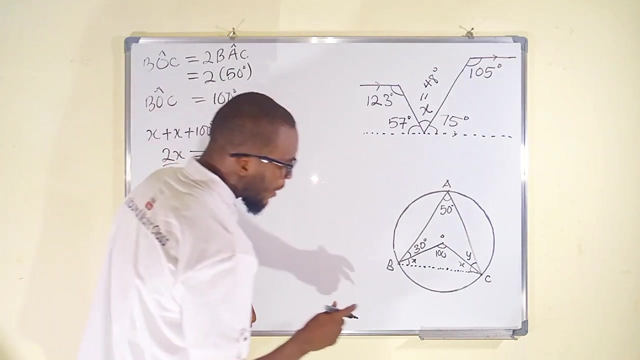 100 to the right and it becomes negative. we have 180 minus 100, which is equal to 80. divide both sides by 2 to obtain the value of X, and X, finally, is equal to 40 degrees. means that each of these angles equals 40 degrees. all right, look at, we have another triangle here, a. 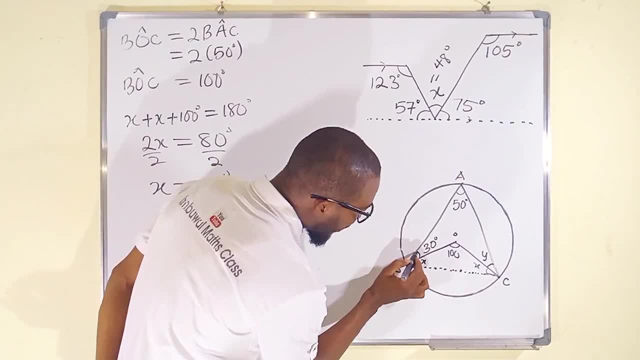 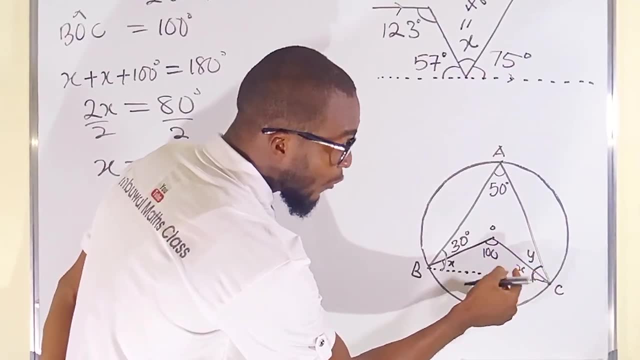 here a, b, c, so the total angle from here to here is going to be 30 plus 40, and the angle here will be x. okay, 40 plus y, and this is 50. if you add all of them together, you shall obtain 180 as well. 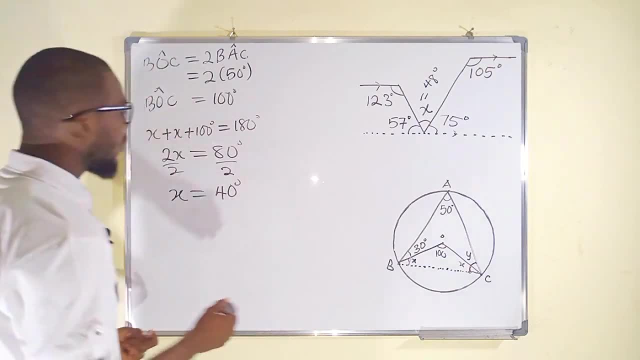 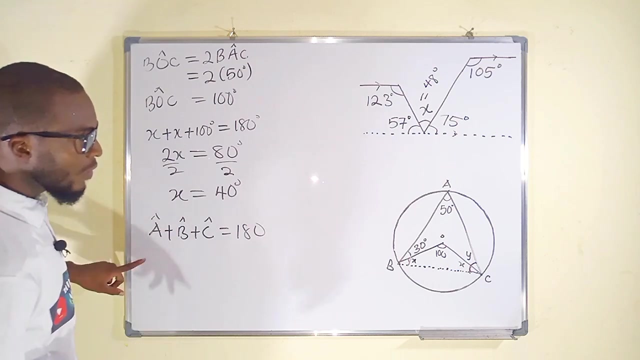 so we can use it to find the value of y. so if we add all of them together we will obtain 180. So we have angle A plus angle B plus angle C is equal to 180 degrees. What is angle A is 50 degrees from the diagram. 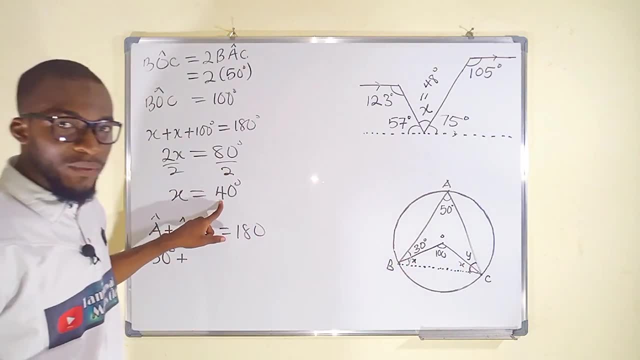 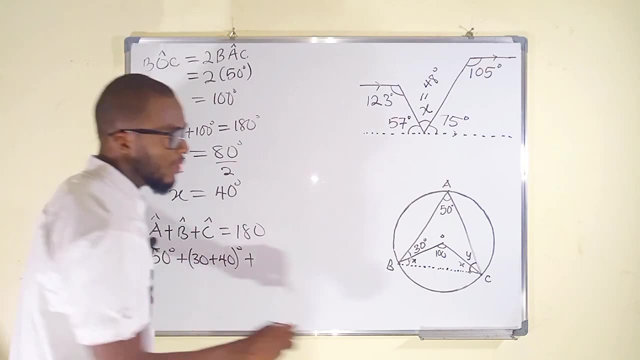 And B is the combination of 30 and X. Remember, X is 40 degrees, So we have 30 plus 40 degrees, plus angle C is the combination of Y and X, But X is known as 40 plus Y, which is unknown. 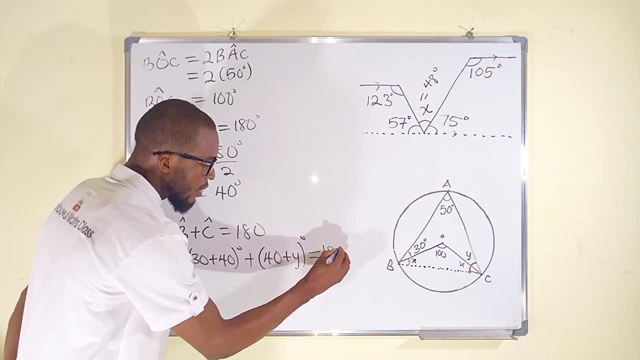 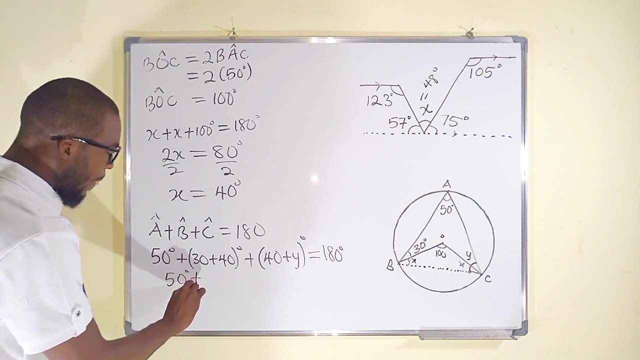 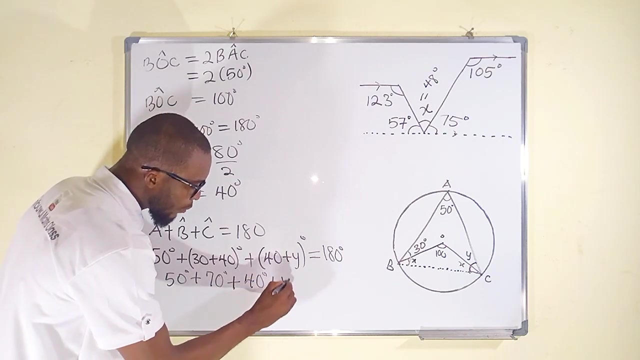 We want to find it And this is equal to 180 degrees. Okay, This and this is 70. So we have 50 degrees plus 70 degrees plus 40. The degrees plus Y which we are looking for, the whole of this must be equal to 180. 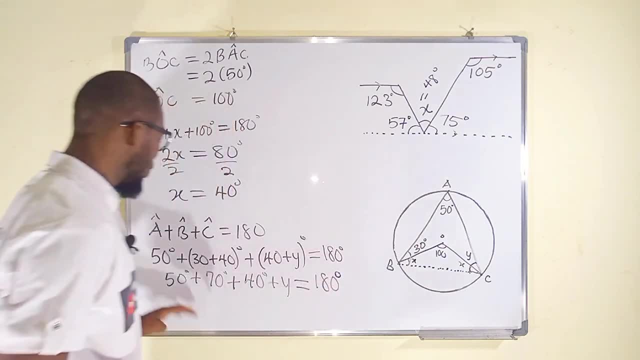 So what do we do to find the value of Y? We want to take all these constant terms to the right And they are going to subtract, leaving only Y to the left. So we have Y, And to the right we have 180.. 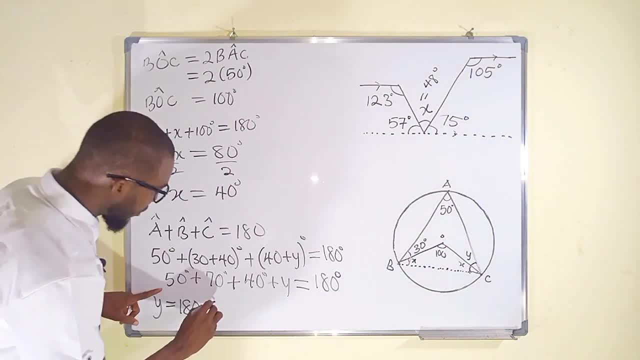 Then we are going to subtract each of these constants, Starting with this. we have 50.. We have 70. And we have 40. All of them in degrees. So now let me use my calculator to subtract all these from 180.. 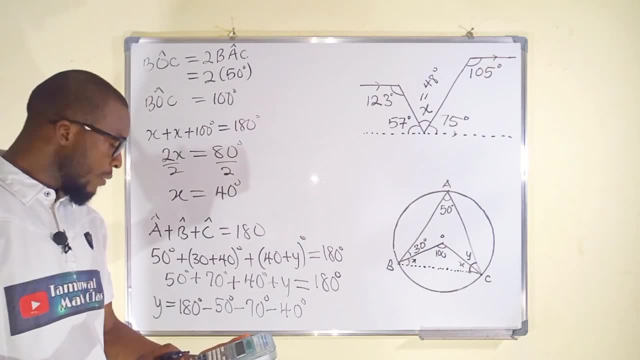 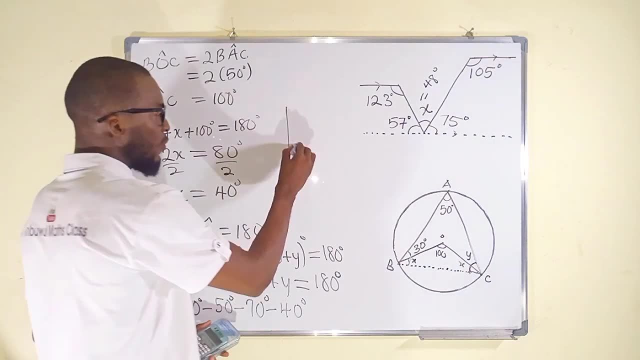 We have 180 minus 50, minus 70. And finally minus 40. And what we have here is 20.. This means that Y is equal to 20 degrees. You can see, this is 30, this is 20.. 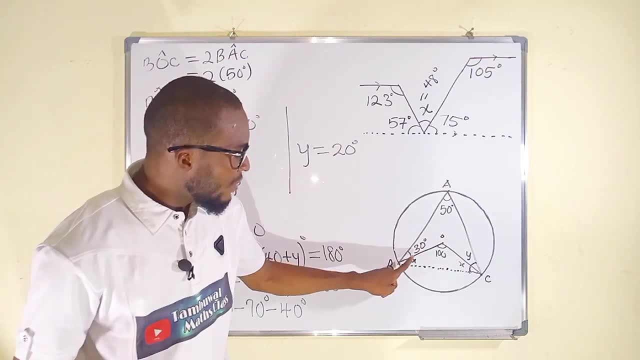 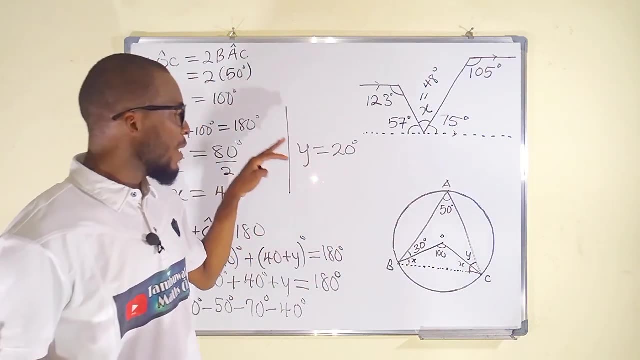 They are entirely different. So if you are thinking that since this angle is 30, this must be 20.. This must be 30 as well, You are wrong. You can see. finally, we are able to obtain angle Y to be equal to 20 degrees. 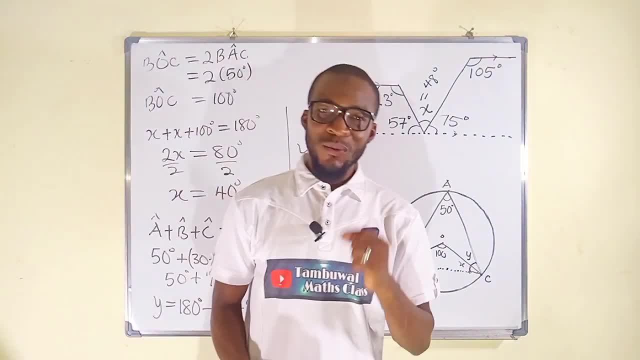 And this is all I have for you today. Thank you for watching. Do have a nice day. 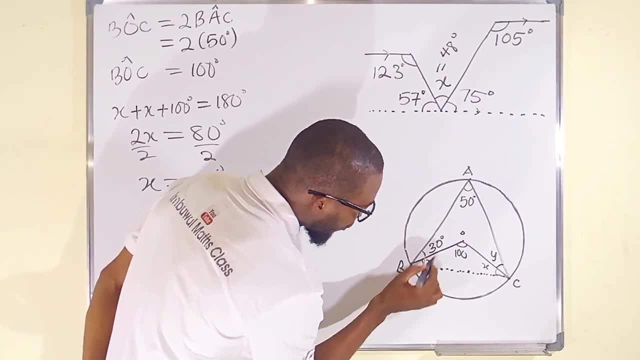 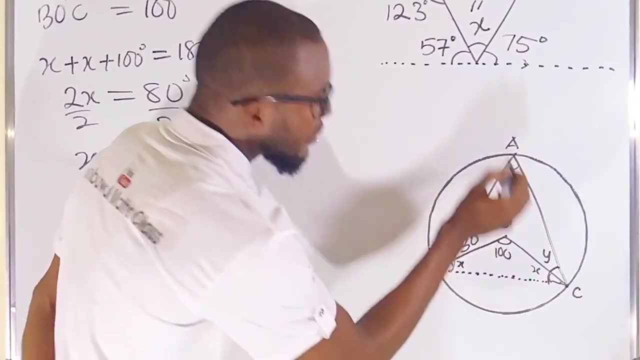 b, c, so the total angle from here to here is going to be 30 plus 40, and the angle here will be x. okay, 40 plus y, and this is 50. if you add all of them together, you shall obtain 180 as well. 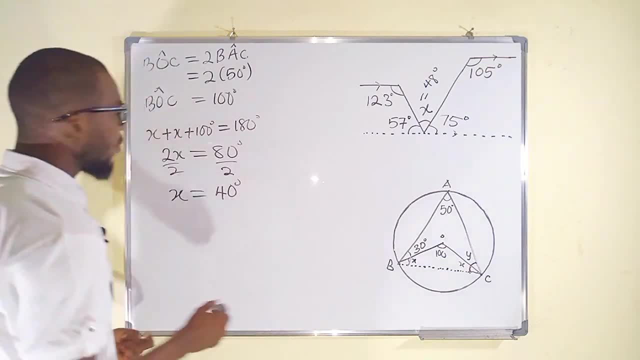 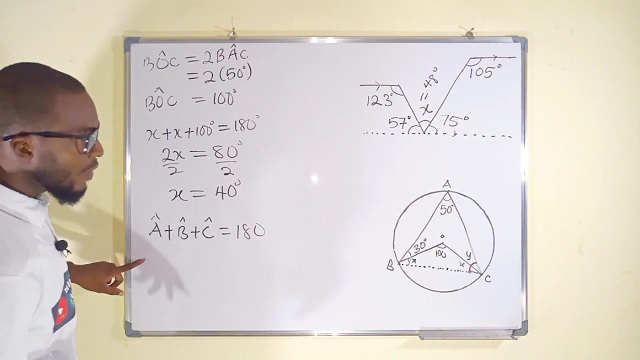 so we can use it to find the value of y. so so we have angle a plus angle b plus angle c is equal to 180 degrees. what is angle a is 50 degrees from the diagram, and b is the combination of 30 and x. remember, x is 40 degrees, so we have 30 plus 40.